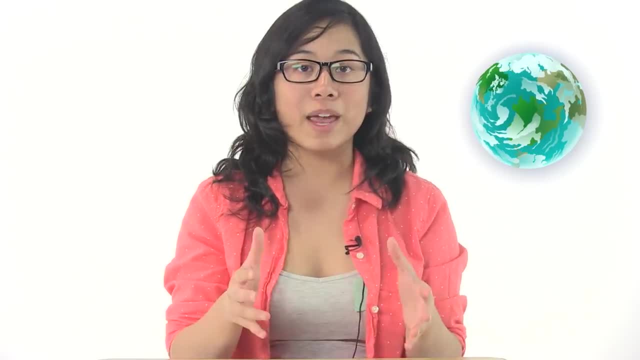 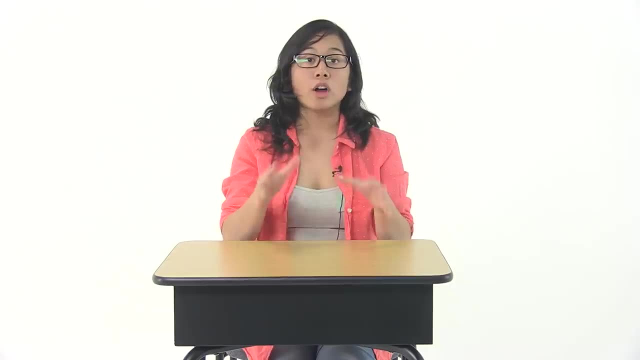 Yes and no Sure. this is what Earth looks like from space, but even though it looks pretty much the same from whenever we view it from afar, once you zoom in on it you can see it's always changing On a small scale. things like moving water shape the Earth's landforms, the natural 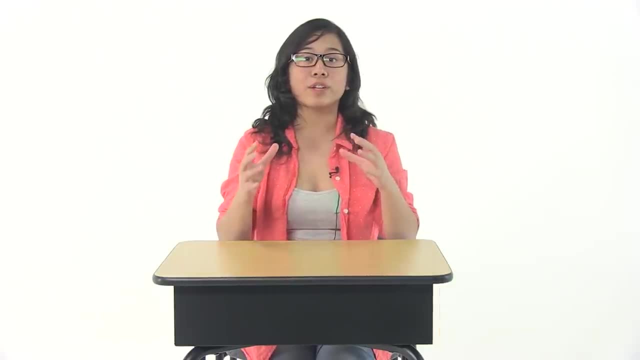 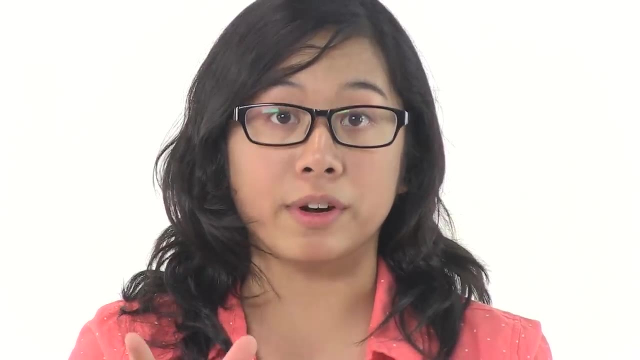 features of the Earth's surface On a bigger scale. the gradual shifting of the Earth's crust is slowly moving even bigger things like the oceans and the continents. So one day our planet will look different, maybe a lot different from how it looks now. 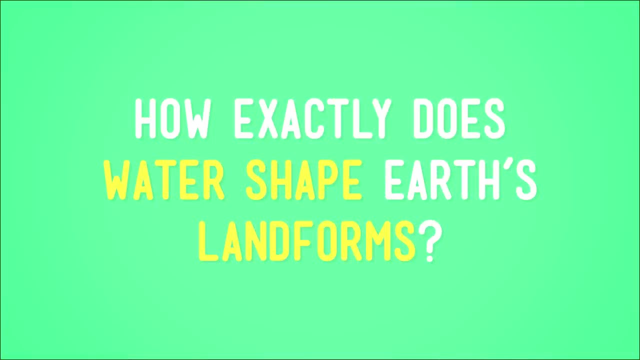 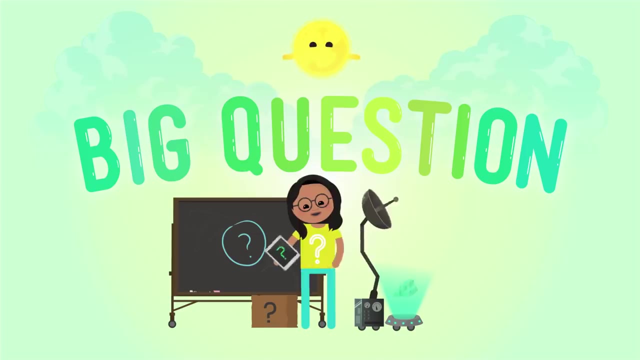 So how exactly does water shape Earth's landforms? Or, to bring it back to the spheres we've been talking about, how does the hydrosphere look? How does the geosphere affect the geosphere? To understand that we need to discuss weathering- I'm not talking about the weather like 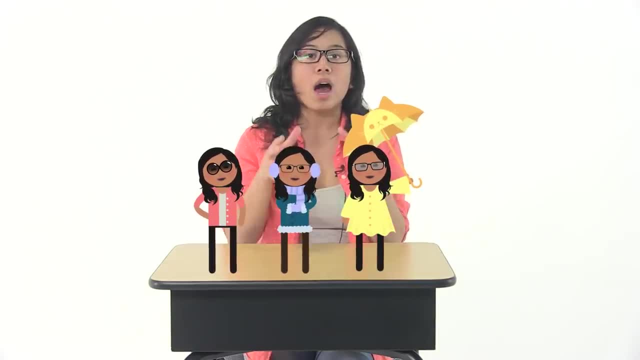 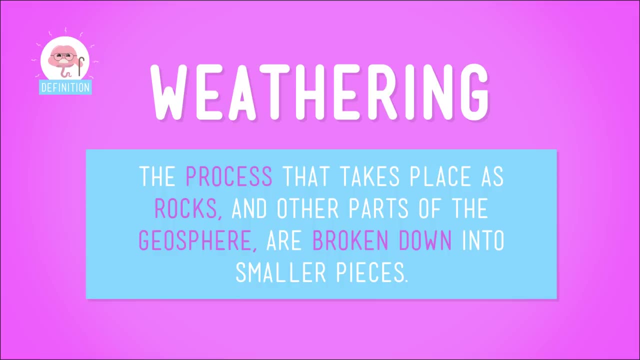 if it happens to be sunny or cold or foggy outside your window. right now. I'm talking about weathering, the process that takes place as rocks and other parts of the geosphere are broken down into smaller pieces. Weathering can be caused by water, air, chemicals, plants or even animals, including us. 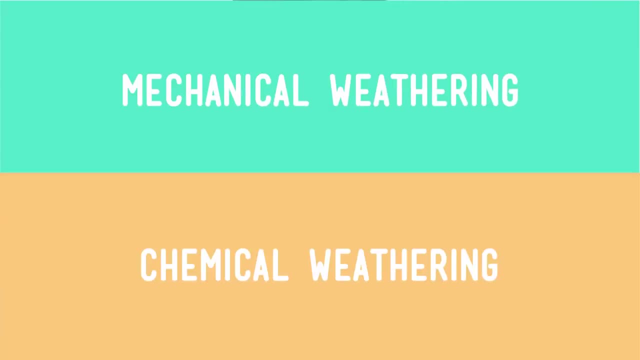 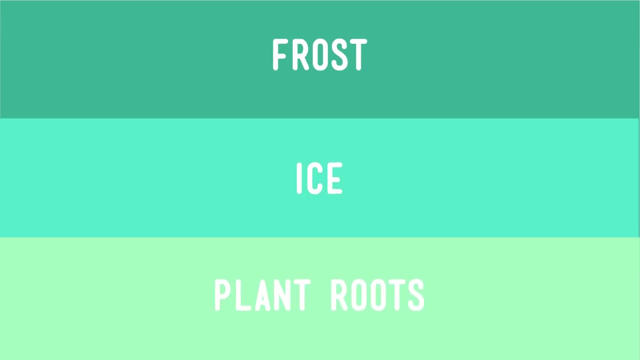 And there are two types of weathering. you need to know about mechanical weathering and chemical weathering. Mechanical weathering is the process of breaking big rocks into little ones. Frost, ice, the roots of plants, running water or heat from the sun can all cause mechanical weathering. 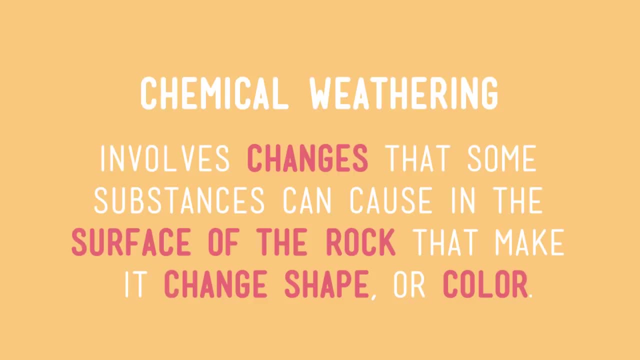 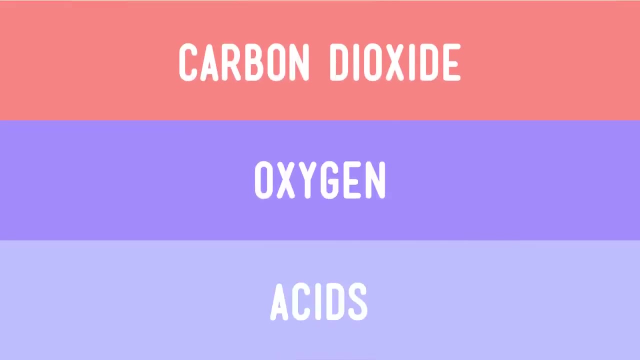 Chemical weathering involves the changes that some substances can cause in the surface of the rock that make it change shape or color. Things like carbon dioxide, oxygen and acids can all cause chemical weathering. And when rocks have been weathered and all broken down and are later moved by natural, 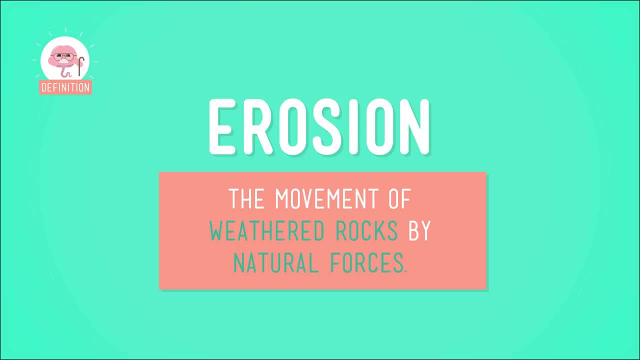 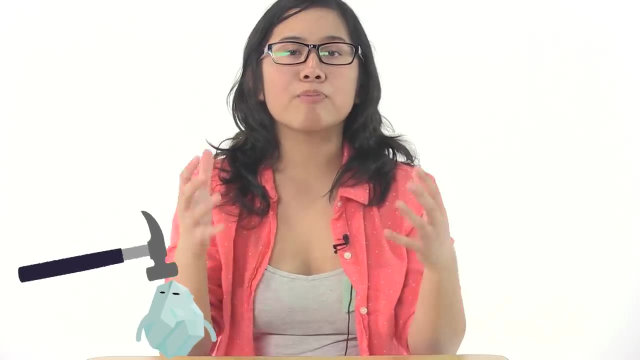 forces like wind, water or ice. that's called erosion. Weathering and erosion sound pretty similar, right? Well, yeah, But not exactly. Think of weathering as the hammer that breaks down the rocks. Erosion is the process that carries those rock fragments away, or put in a way we're 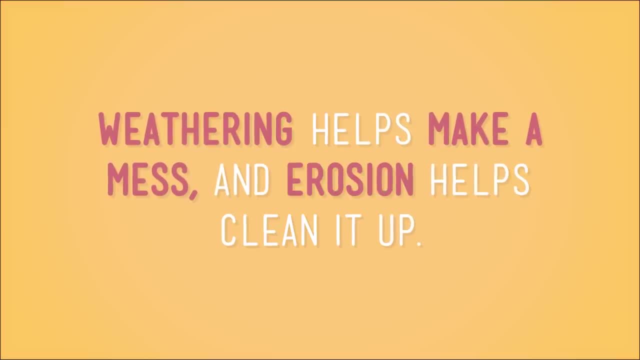 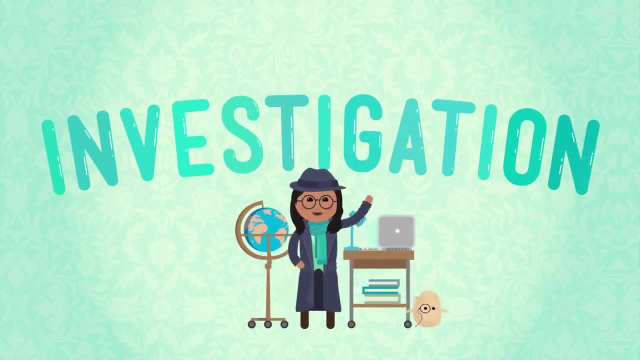 all familiar with. Weathering helps make a mess and erosion helps clean it up. Let's take a trip to the beach to see what part the hydrosphere plays in weathering and erosion. This is a picture taken from space of the coastline of Massachusetts in the northeastern.